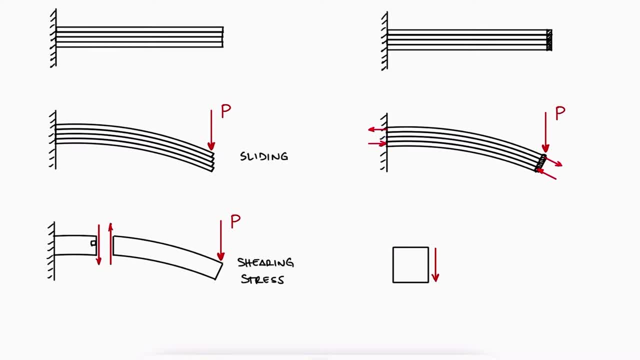 performing a cut of the cantilever just to the right side of the element and since we know that the element is not moving down, there will be an opposite reaction in the opposite side. and since the element is not rotating, there will be reactions on the top and the bottom faces that. 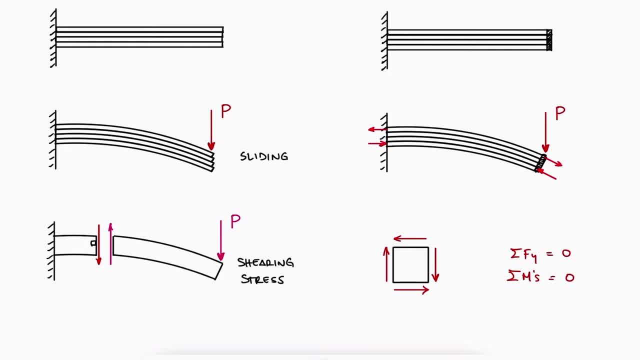 counteract the rotation caused by the vertical vectors. Alternatively, we can start by using the plank simile to see that the plank above it would want to move the top face towards the left, to return to the original position And with the same reasoning from before, knowing that the element is 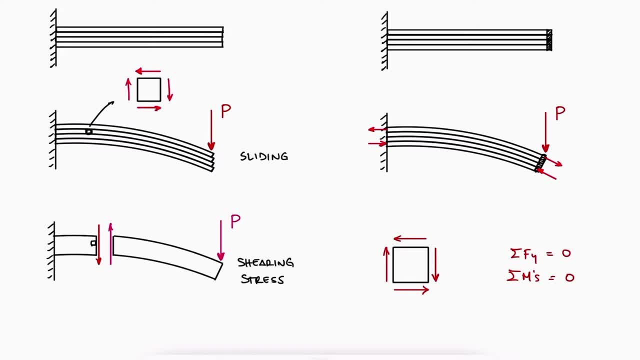 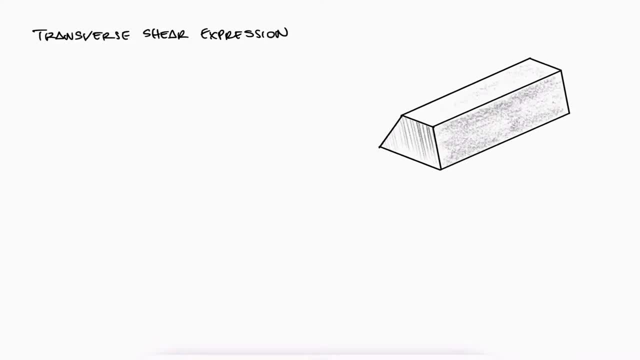 not translating nor rotating. you can get the other three vectors By looking at a beam of a constant cross-section area, and that cross-section area doesn't need to be a trapezoid, it can be any shape, but I use the. 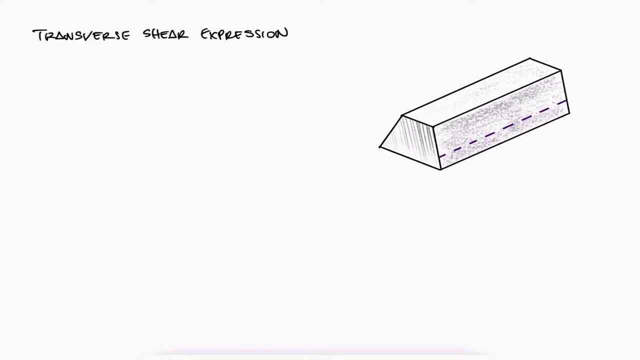 trapezoid instead of a rectangle, so that the neutral axis is not right at the center. we can subject it to some distributed loads and point loads to study the shearing stresses that appear on the horizontal planes. If we take out a rectangular chunk of the beam by performing two 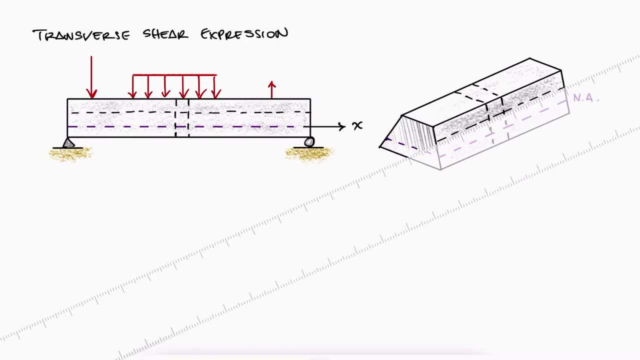 cuts along the x-axis and another one perpendicular to the y-axis. we can analyze the external forces that this sliced chunk is subjected to Because of the bending that the external loads and couples generate on the beam. we know that anything above the neutral axis will be subjected to compression and anything below the neutral axis 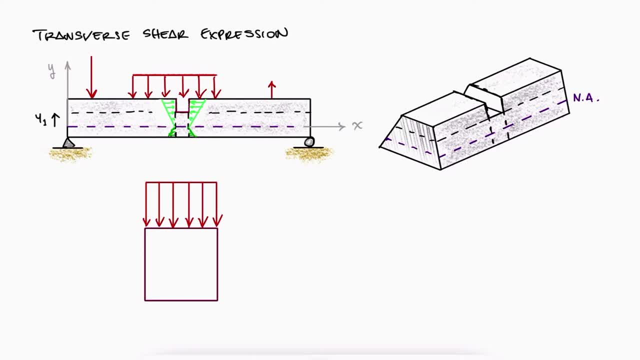 will be subjected to tension. Since our point of reference is found at y1, above the neutral axis, the chunk of beam we're taking out would be subjected to that linear profile of compressive stresses. There will be some vertical reaction forces at the cuts and a horizontal reaction from. 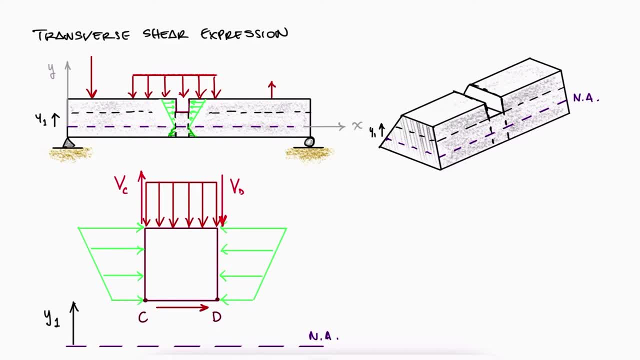 the contact between the chunk and the beam. This horizontal reaction is usually referred to as delta h. The shearing stress that the shaded area in yellow would be subjected to would be that shear force, delta h, over the shaded area in yellow If the slice perpendicular to the x-axis is small enough. 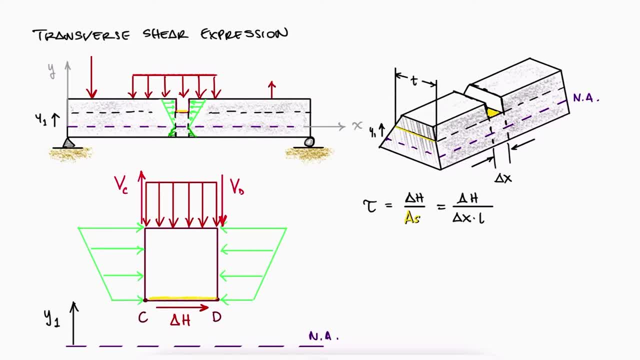 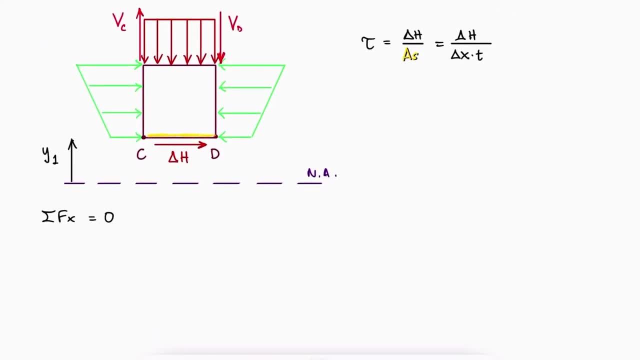 this area can be calculated as delta x times t, But let's focus on the force for now. A sum of forces in the x-direction, which we know has to be equal to zero since the element is not left or right, would have a positive delta h and the total forces that result from the compressive 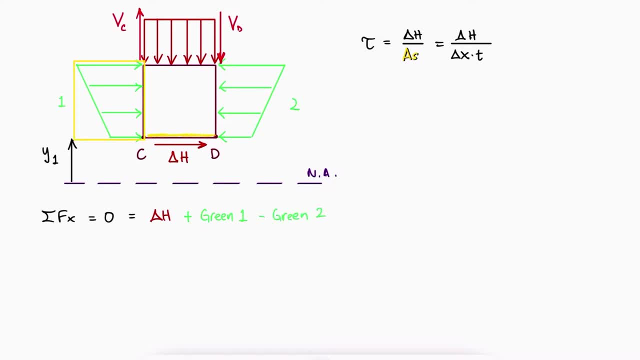 stresses. The total force affecting the left face would be equal to the value of the stress which varies and increases along the y-axis times an infinitesimal area dA integrated from y1 to the top of the beam. The total force on the right face would be the same expression with sigma d. 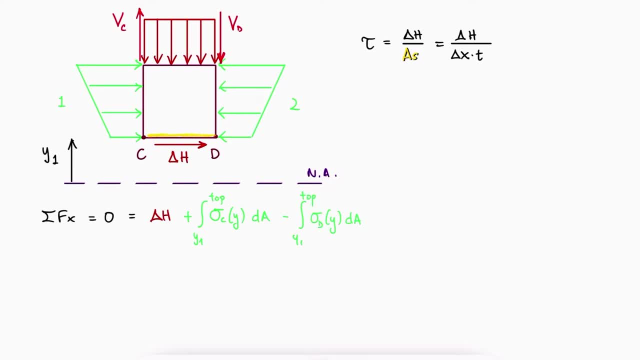 instead of sigma c, Since we know that the normal stress sigma is the normal stress due to bending. sigma can be substituted by minus my over i. The moments at d and c are different because we know that the moments can vary along the x-axis But since the moments are constant along the y-axis. 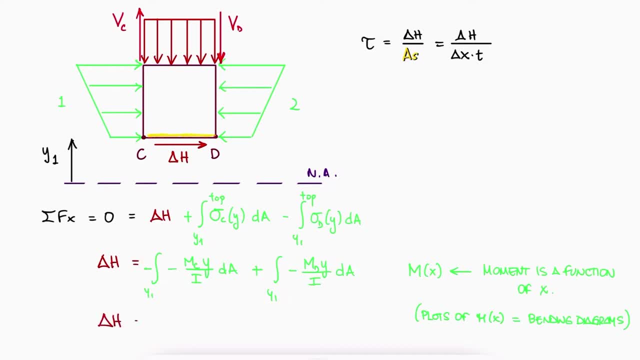 which is what we're integrating them over. both the moments and the second moment of area i can be taken outside of the integral. Delta h is therefore equal to delta m over i times what we call the first moment of area q. Notice that our point of view is this. 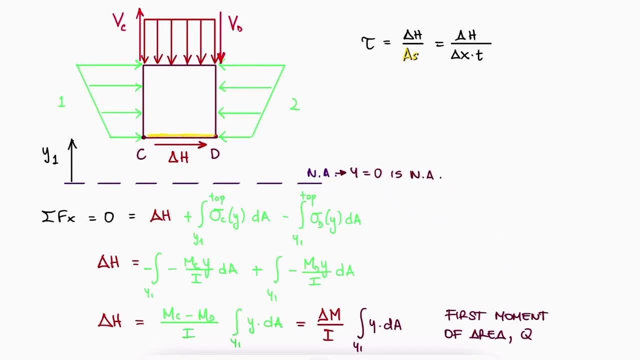 of reference for that integral is the neutral axis, as we are integrating from y1,, which is a distance that has the neutral axis as the reference, and the area that we care about is from y1 to the top of the beam. This first moment of area is similar to the second moment. 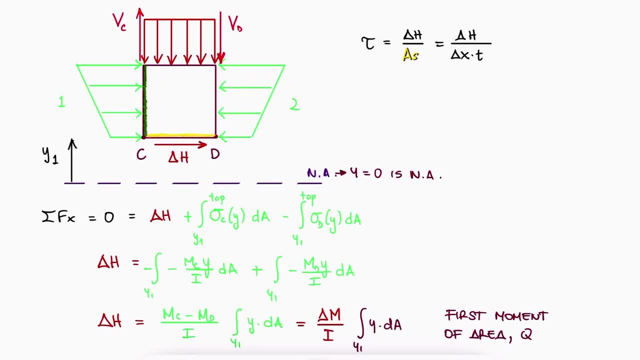 of area that we covered in the main bending and torsion videos links below. The only difference here is that it's not y squared or r squared, it's just y, And, of course, that the integration limits are different. This first moment of area Q actually refers to the first moment of area. 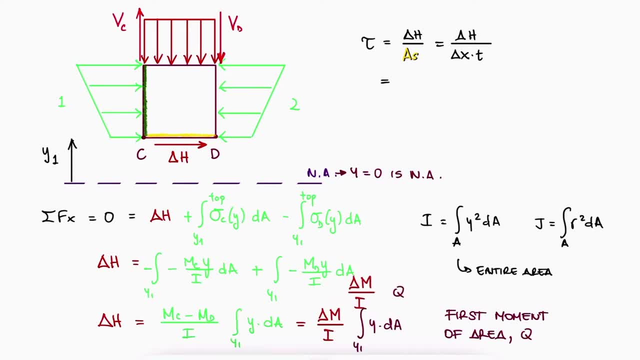 about the neutral axis. If we now go back to the shearing stress expression and substitute what we found for delta H, and since we can identify that when the slice along the x-axis is very small, the expression delta M over delta x becomes dM dx, which is the derivative of the moment with. 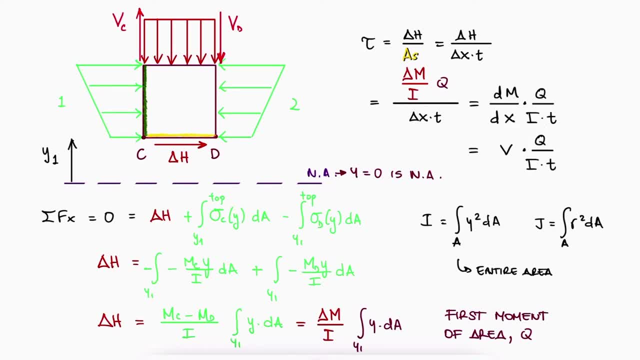 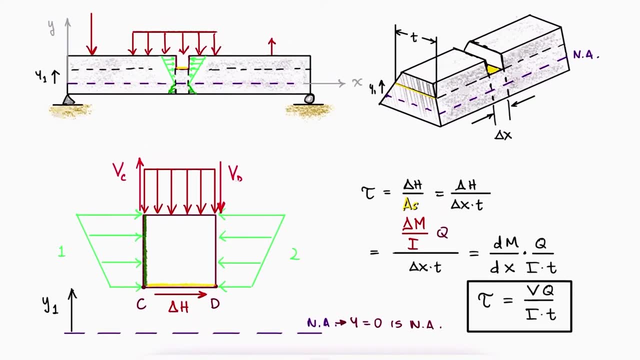 respect to x or just the shear force V, if you remember about the moment and shear relationships. Now let's look at the shear force V. This is the shear force V, which is the shear force of the beam. Link to a two-minute video on that is down below The first moment of area Q, which we already. 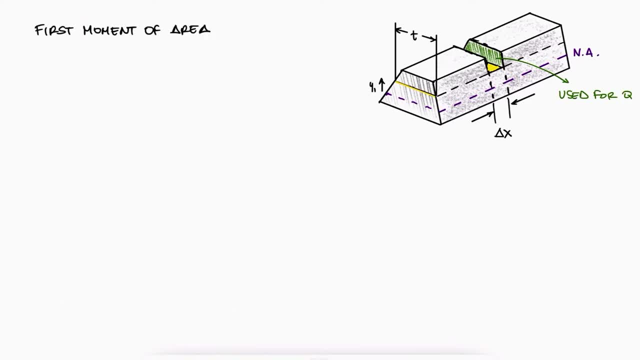 know is referring to the green shaded area, is in general calculated as the shaded area times the distance from the neutral axis to the centroid of that shaded area, The dimension T. that refers to the thickness of the cross-section area for the horizontal plane for which we're trying to find 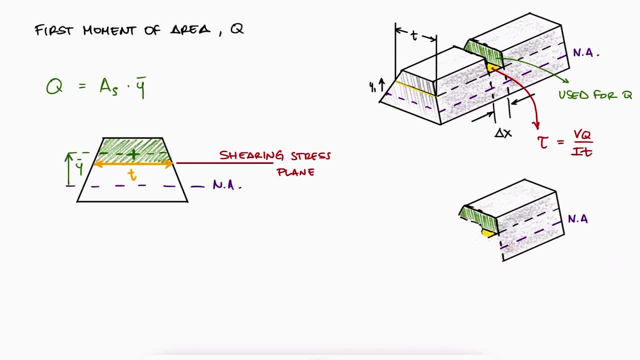 the shearing stress is always a dimension that is perpendicular to the internal shear force V. This is very important to know when you're trying to calculate the transverse shearing stress of a component that is subjected to shearing forces V that are not vertical, The plane from which we would be 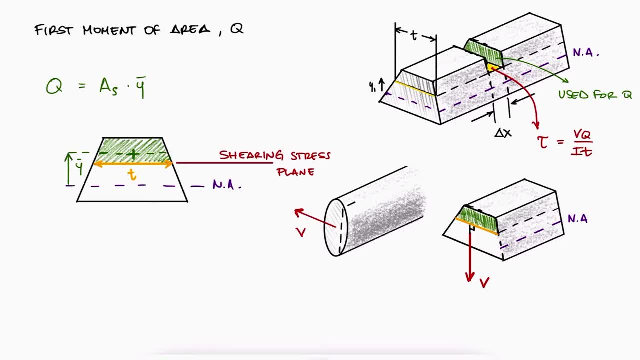 interested in calculating a shearing stress needs to be perpendicular to the shear force V, and so will the dimension T. The shaded area for Q in this case would be: what is on the right or the left of T, Since the second moment of area I came from substituting the normal stresses due to bending. 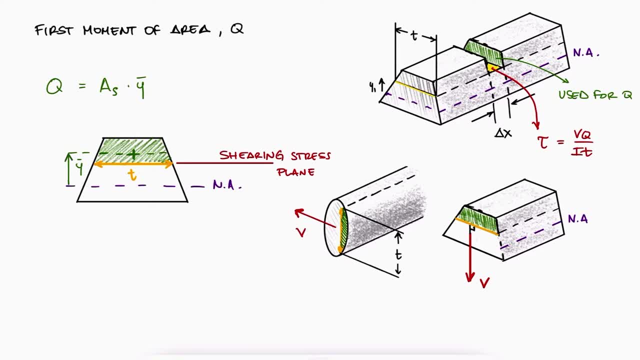 and not something specific from the cuts we performed. the shear force V would be perpendicular to the shearing stress of the component that is subjected to the transverse shearing stress. This second moment of area is the regular I that we would calculate for a bending stress. 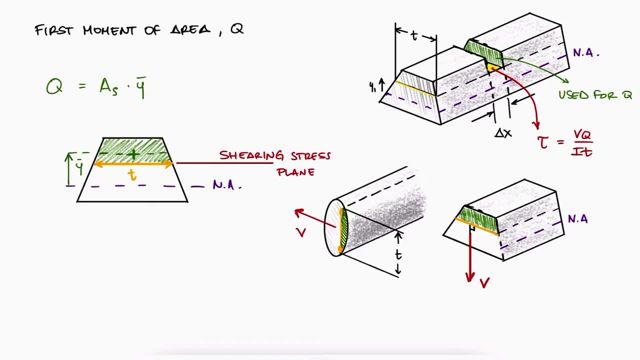 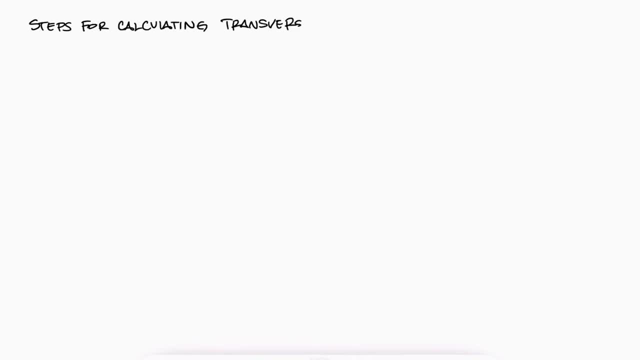 This means that I is not the second moment of area of the shaded area, it would be that of the whole cross-section area. So, in general, when we're trying to find the shearing stress due to transverse shear of a beam at a specific location of the beam, we need to find four variables. If the value for the shear 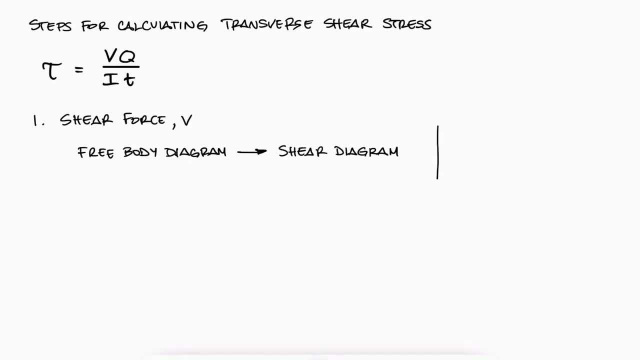 force V is not given. the shear load will generally be found through the use of a shear force diagram. If the location along the beam where we're trying to find the shearing stress is given, then we find V for that value of X. If we're trying to find the maximum shearing stress along 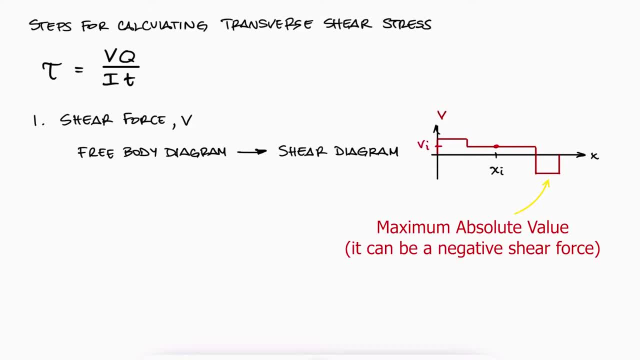 the beam, then the location of the maximum transverse shear stress will be the value for X along the beam for which the shear force shows a maximum value. The thickness T will depend on the Y-location of the horizontal plane when looking at the cross-section area. 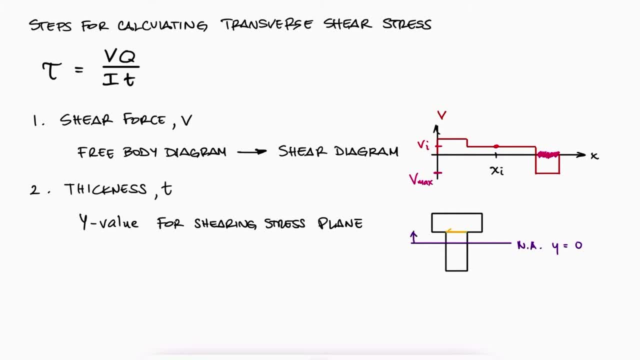 Locations of interest can be glued, soldered or even welded surfaces, since the maximum allowable stress properties there would be different, and usually lower, than the rest of the material. The first moment of area, as explained earlier, will be the shaded area above or below the plane of interest where T was drawn. 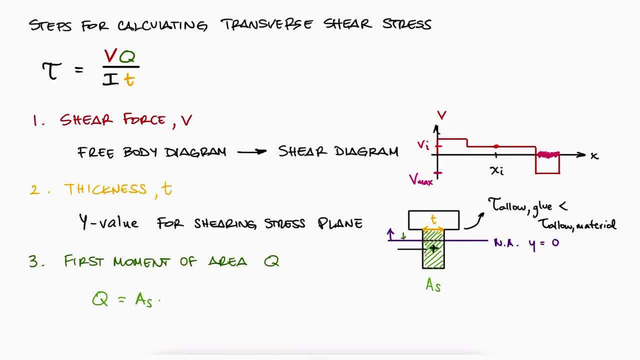 times the distance from the neutral axis to the centroid of that shaded area, And it doesn't matter if it's the area above or below that plane. you will always get the same result for Q. And finally, just like we also stated earlier, 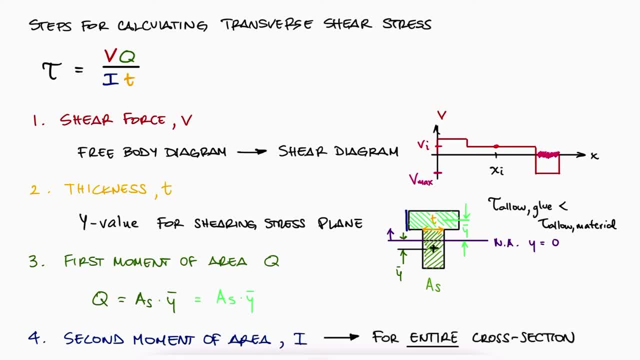 the second moment of interest will be the area above or below the plane of interest where T was drawn, times the distance from the neutral axis to the centroid of that shaded area. Let's take a look at a simple example where we put what we've learned today into use. 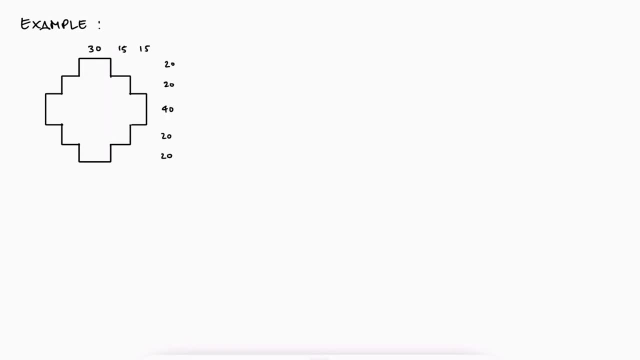 And if you want to check out more complex examples, including finding the location of the maximum shearing stress, make sure to check out the links to those 2-3 minute video examples. in this video's description, Given a beam made out of 6, 2.3 meter long, 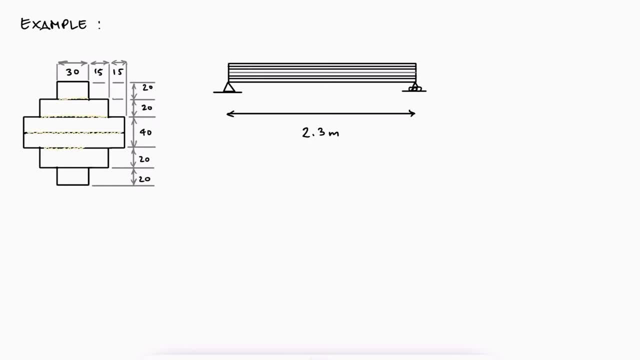 planks of the same material glued together and subjected to a vertical point load. will the glue between the top plank and the rest of the beam hold if the maximum allowable shearing stress for that glue is 10 MPa? Remember to try solving this problem on your own before continuing. 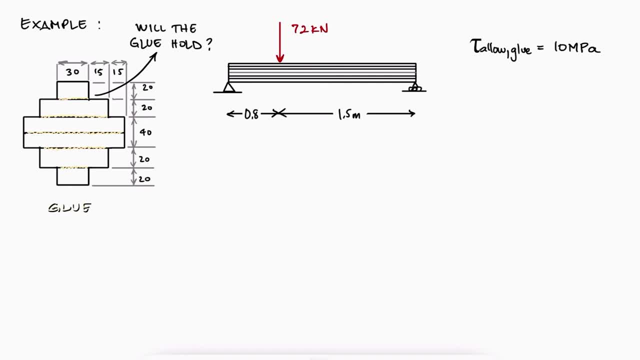 to watch the solution in this video To know if the glue will hold. we will calculate the transfer shear stress at the location of interest, which in this case is the location of the glue between the top plank and the remainder of the beam, And if the stress is higher. 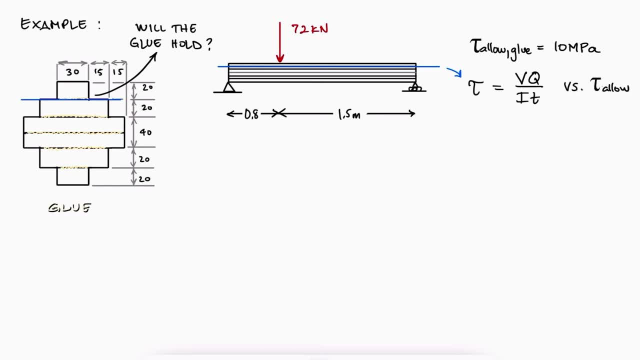 than the allowable shearing stress of the glue. we know it would fail. The maximum shear force V can be found if we draw a free body diagram, write a sum of moments about C and the sum of forces in Y and find the reaction forces at A and C to draw a shear force diagram. We see that the maximum 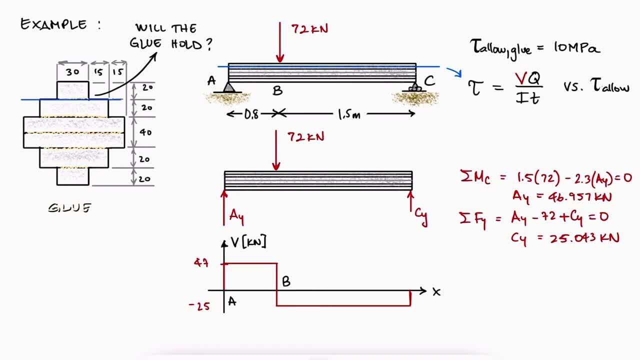 shear force V occurs anywhere between A and B and that its magnitude is almost 47 kN. The first moment of area Q is the shaded area above the location of interest times the distance from the neutral axis to the centroid of that shaded area, Since the neutral axis is located right at the center due to the cross-section being symmetric. 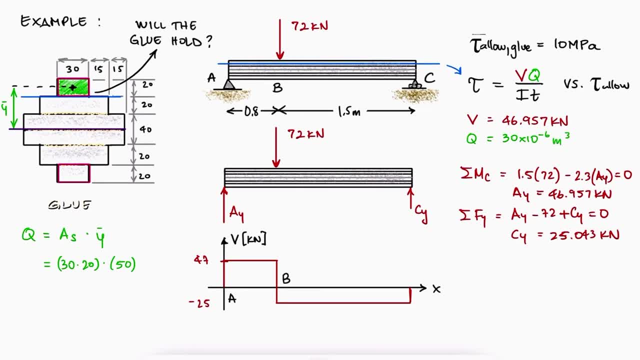 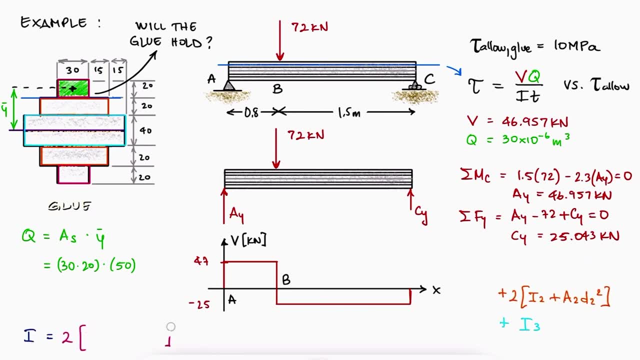 this distance is 50 mm. The second moment of area I can be calculated using the parallel axis theorem and adding three I's together. If you need a refresher on second moments of area or the parallel axis theorem, I'll leave two links to videos where these are explained in detail in. 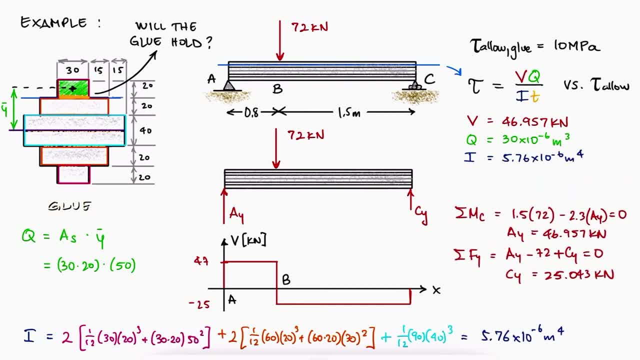 a very short amount of time. If you want to learn more about the parallel axis theorem, click the link in the description. The thickness T at that location would be the base of the top plank. Substituting these values, we find a transverse shear stress of 8.15 MPa.